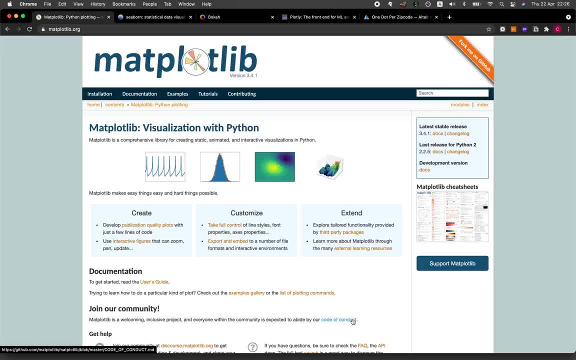 is, of course, Matplotlib. So Matplotlib is probably one of the oldest data visualization library for Python And it has a wide range of functions for you to visualize data in all sorts of ways And so in all of the websites for the five data visualization libraries, all of them. 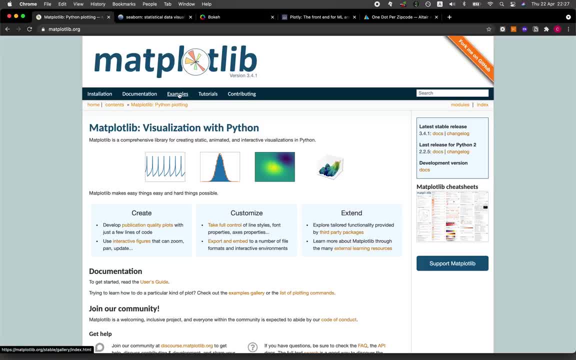 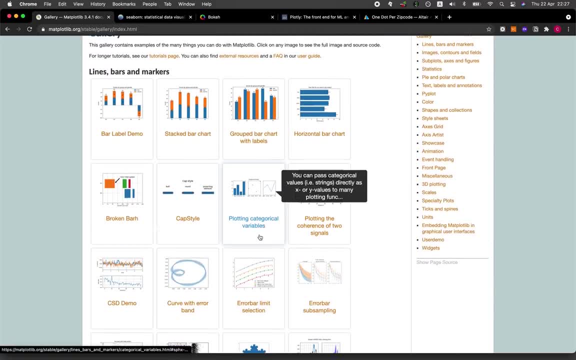 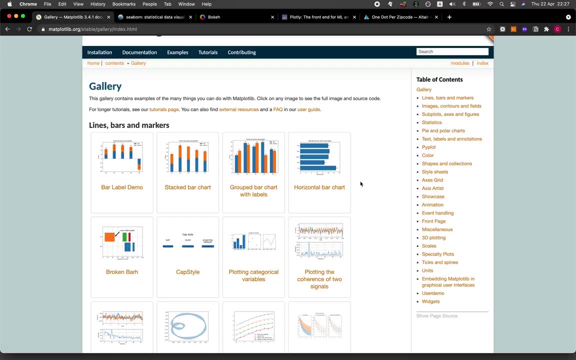 will have a gallery, And so, for example, if I click on examples here, I will see all of the possible plots that I could make using Matplotlib, And so on the right hand side, you can see a table of contents which you can click and it will jump to the one that you want. 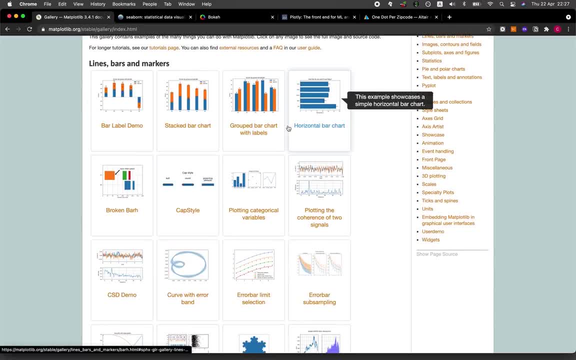 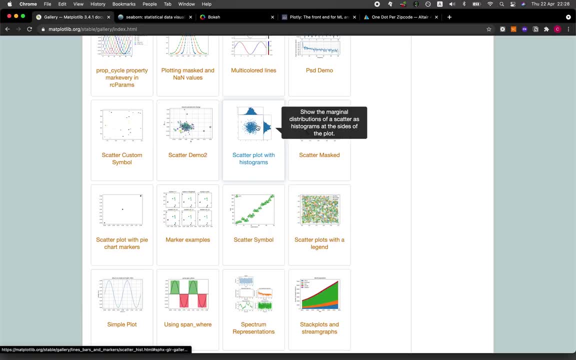 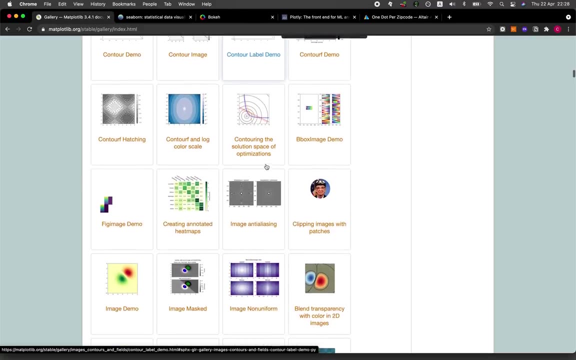 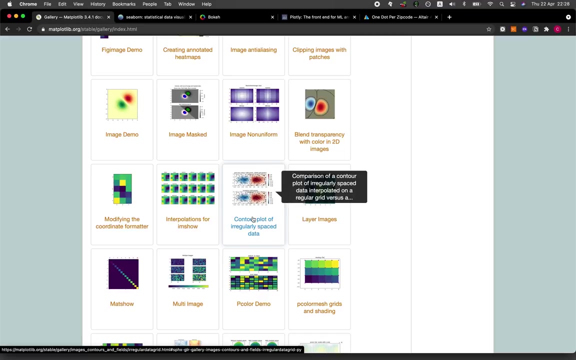 So here we're just going to scroll down. So it has bar charts, lines, even histogram and scatterplot fused into one. Okay, so this is contours and also for images. So contour plot is pretty good in allowing you to visualize three dimensional data whereby the X 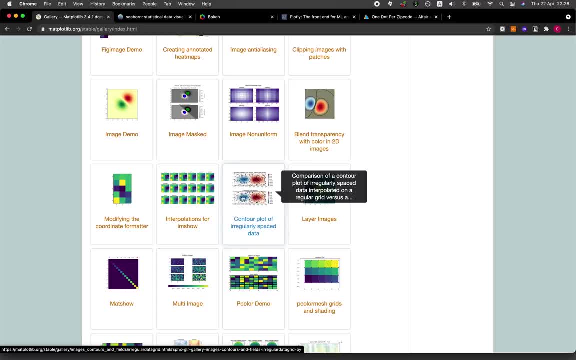 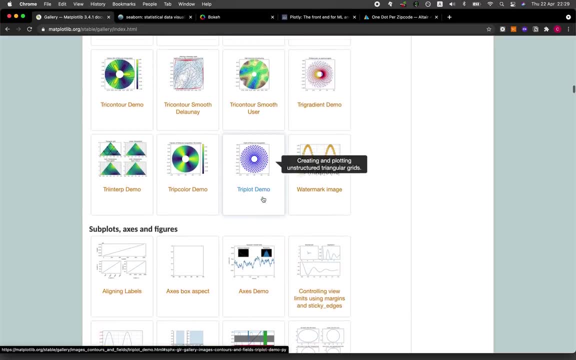 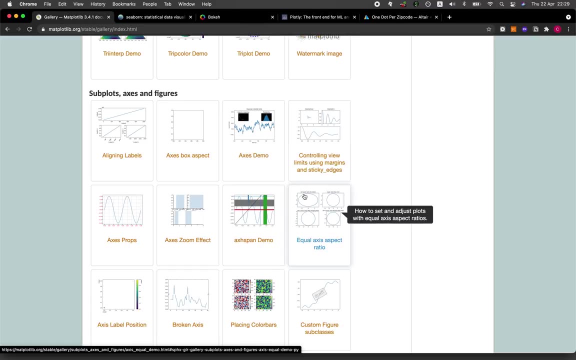 and Y are indicated here, and then the Z dimension is indicated by the data samples that you see, along with its corresponding colors. And then this is for customizing the various axes, labels, making a multi plot figure, adding text to the image. 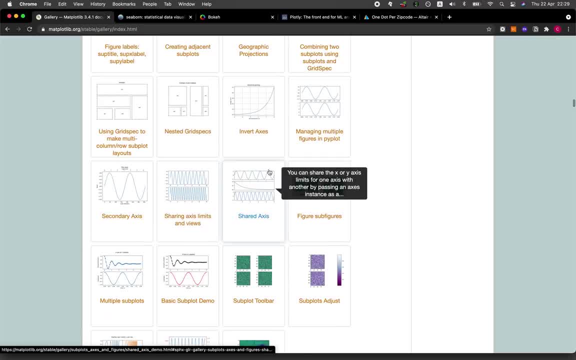 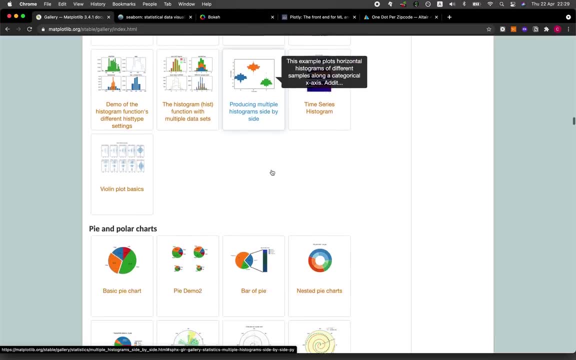 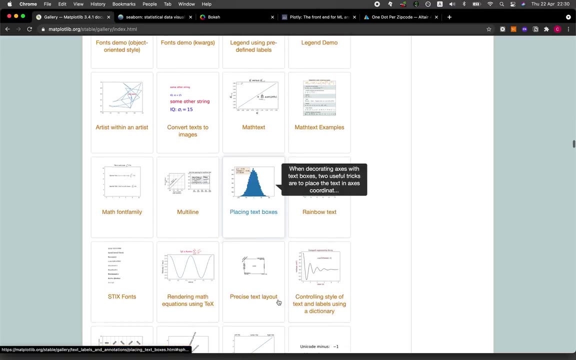 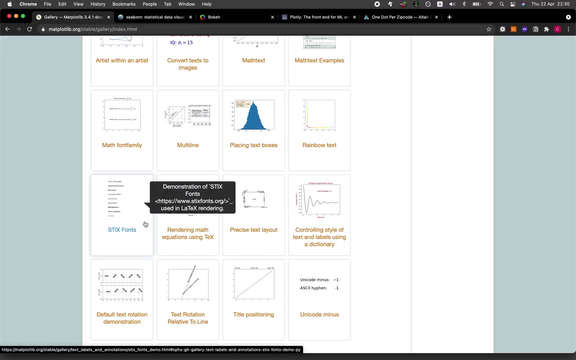 plot, arranging the image plot as a grid, And also a lot of plots for statistics. And of course there's the pie plot and the polar chart as well, And they provide you some examples on how to create all sorts of annotated image plots: how to add latex into the image plot here. 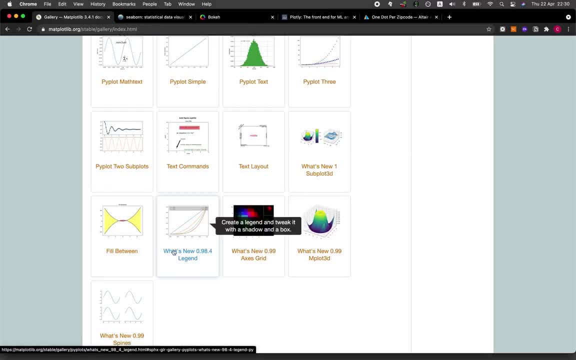 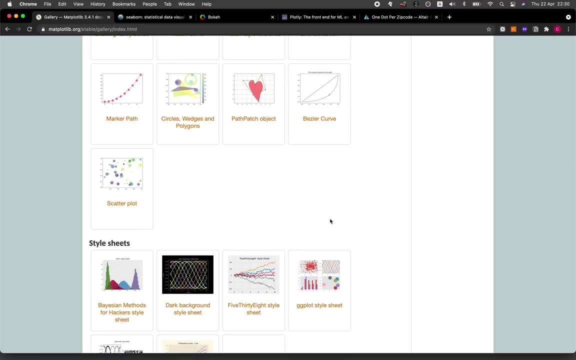 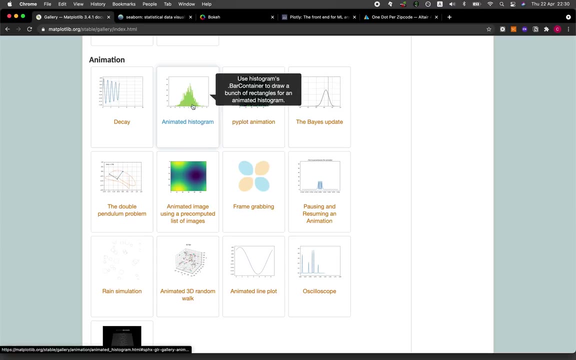 Okay, so all sorts of annotation examples, and also how to work with colors in the plot that you're making, And so, as you can see, there's a lot of things that you can do with Matplotlib, Even animated histograms as well. 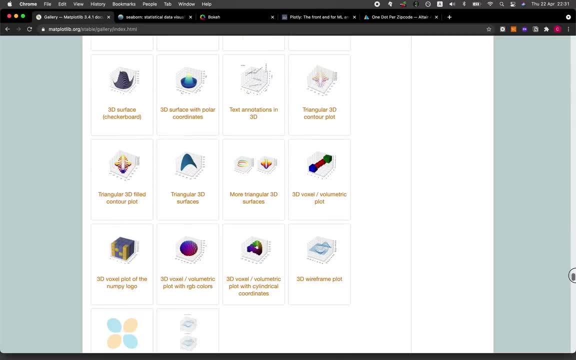 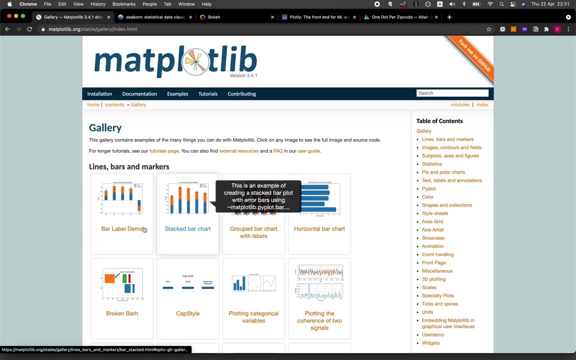 So I'm just going to scroll it, because there's so many plots, as you will see here, even 3D, here 3D, contour plots. Okay, actually, if you are interested in any of the plots here, just click on it. 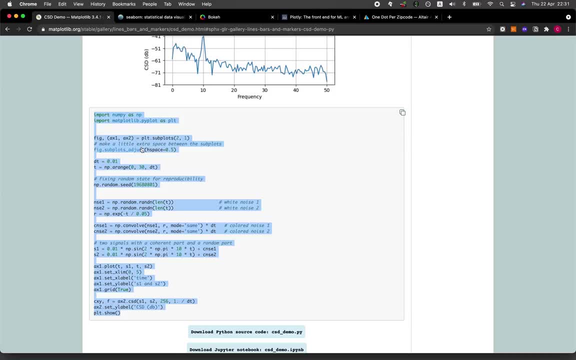 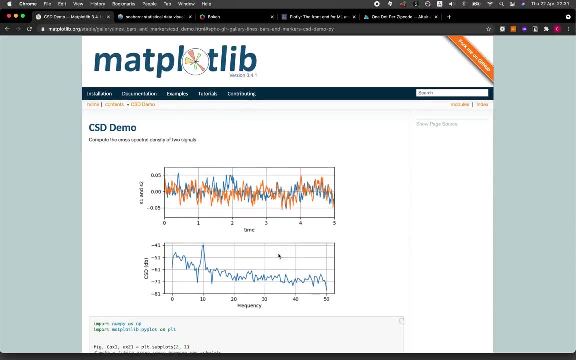 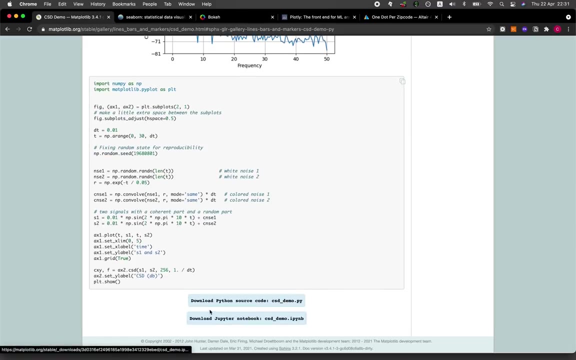 And then, and so it will provide you the example code to get you started in creating the plot indicated here, And so I would normally just shop for the image plot that I like, look at the example and then replace the example data with my own data, And you could also download the Jupyter Notebook of each of the image plots to your 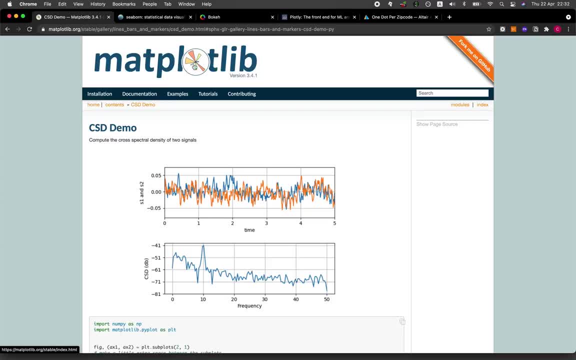 own computer and customize. Okay, so, this is pretty much it. Okay, so, this is pretty much it. Matplotlib, and it's a pretty good library for data visualization. So let's hop on to the next one, Seaborn. 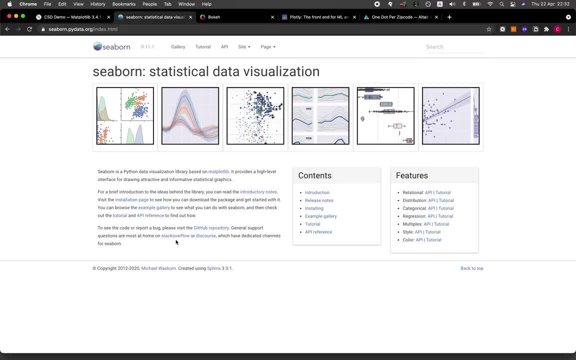 So Seaborn, in my opinion, looks a bit better than Matplotlib. I think it's because of the color scheme, in that it resembles that of the ggplot2.. As you can see here, the coloring scheme looks amazing. So let's have a look at the gallery. 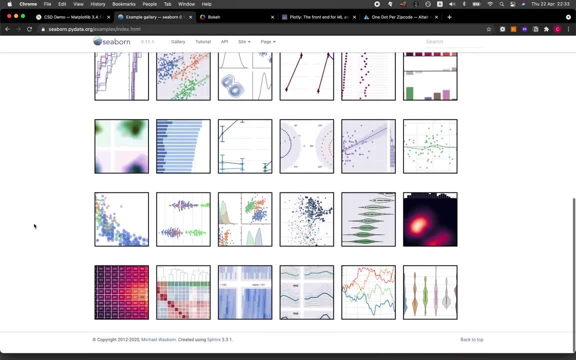 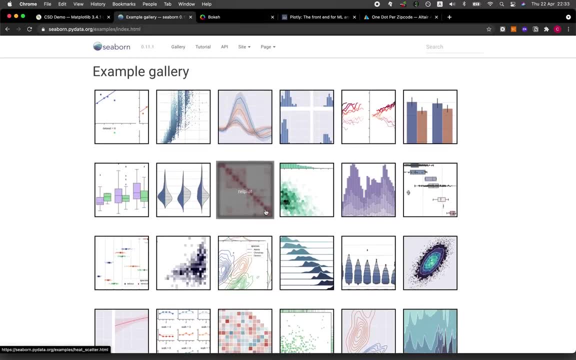 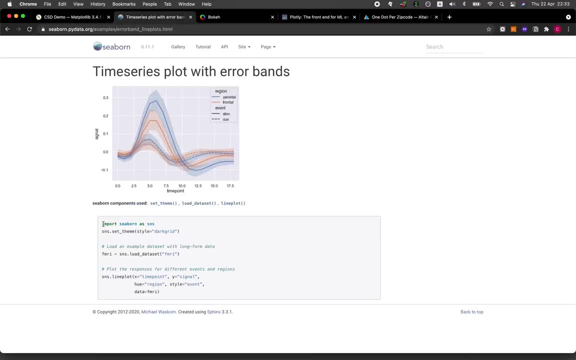 So the gallery is not as extensive as that of the Matplotlib, But it does have quite a few standard plots that you would need. Let's click on one of them And, similar to Matplotlib, it provides you the example code that could get you started to reproduce this. 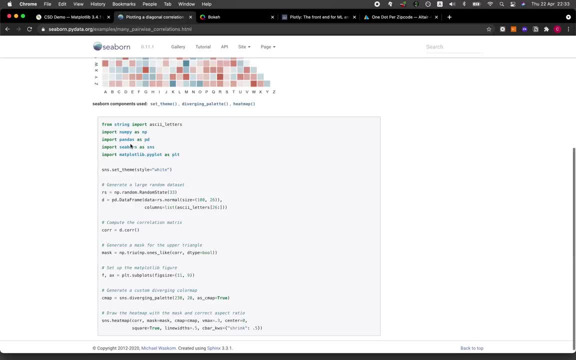 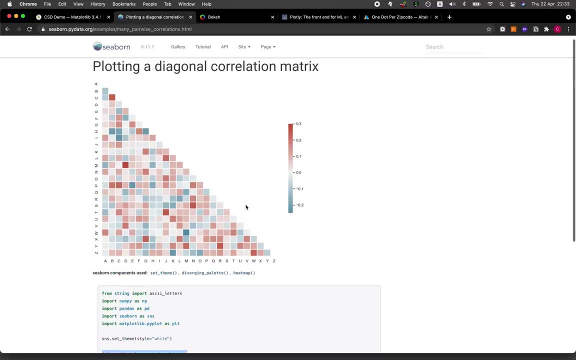 If you're interested in a heat map, you can make it. Just follow this example, just copy and paste it into a Jupyter Notebook and replace the example data with your own data, But also to compare and have a look at their own data sets and your own data set. 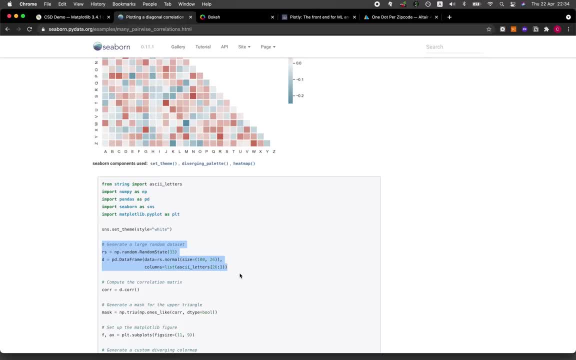 Are the shapes similar? If not, then you have to reshape your data so that it resembles the one in the example here, so that it could plug and play and work with the plots from the example, Right? So there's quite a lot of things that you could do here. 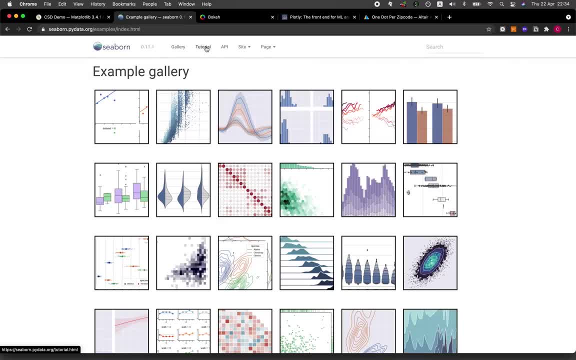 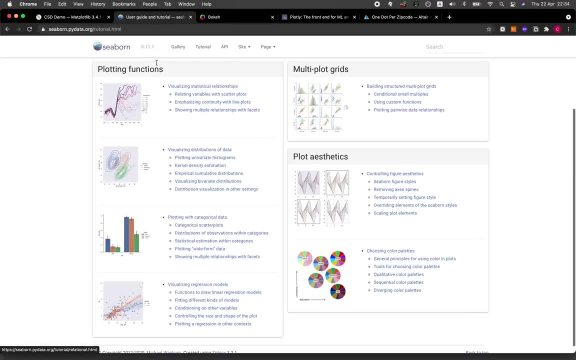 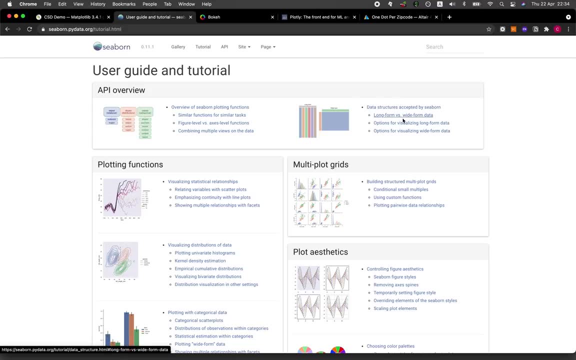 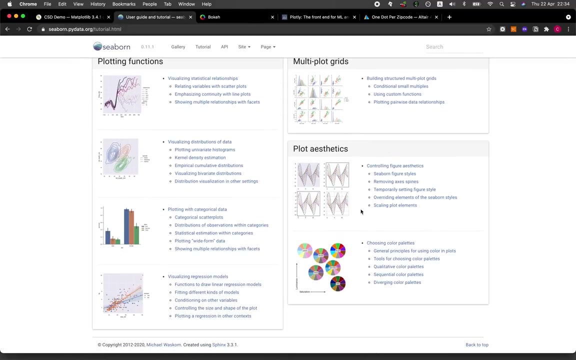 And the great thing is, they also provide the tutorial as well. So let's click on that, And they did a pretty good job in categorizing the tutorials Into making the basic plots, making a multi-plot grid, and also to take a look at some of the data that it accepts, whether the data is in the long form or in the wide form, and also to customize the various aesthetic of the plot. 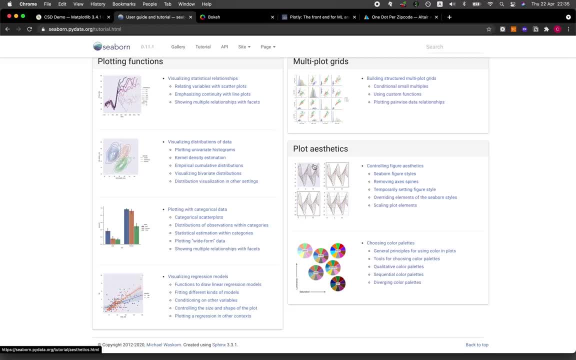 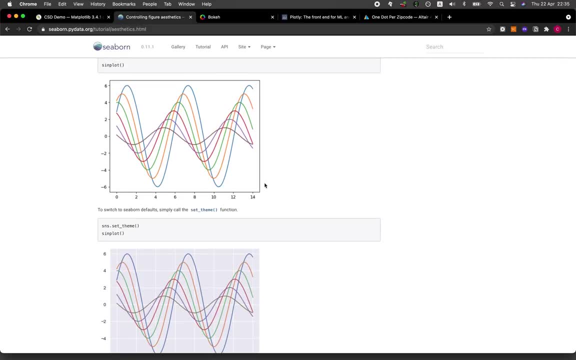 Like, for example, by default, you will see that it provides you a gray background like this one, but you could also make it into a black and white right, like with the black outline here and the white background, So without the major grid. 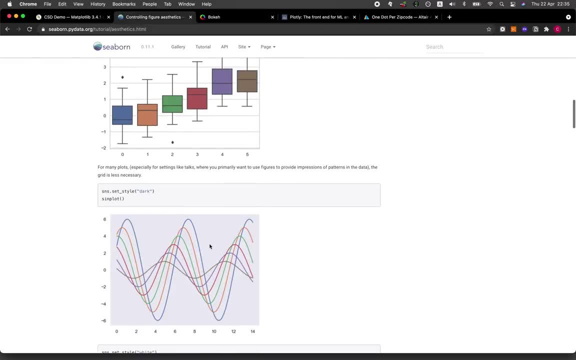 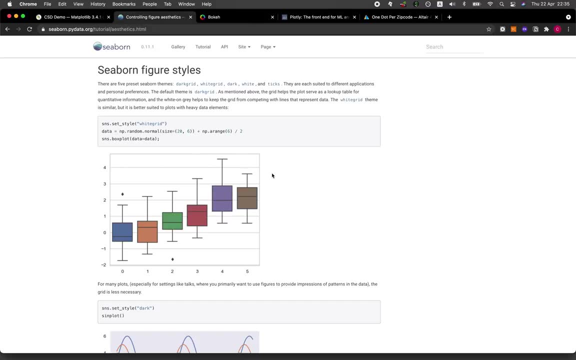 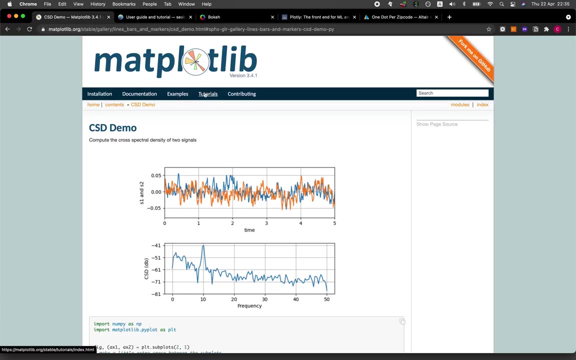 Minor grid as shown here, just a plain gray background or a plain white background, or even a white background with a grid line, a horizontal grid line. Okay, Let's go back and have a look at mapplotlib for a short moment, And it also has tutorial session as well. 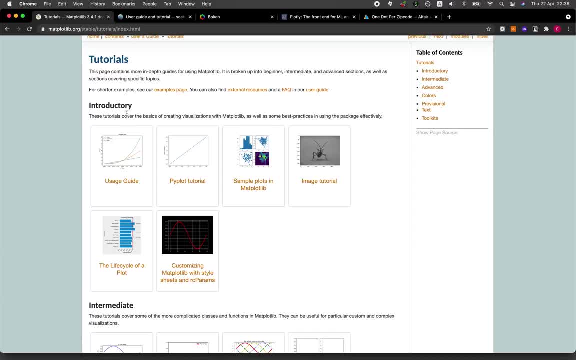 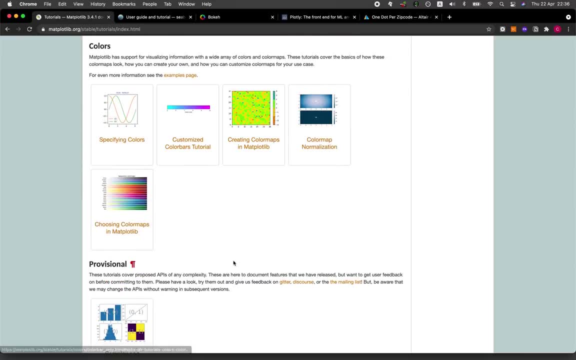 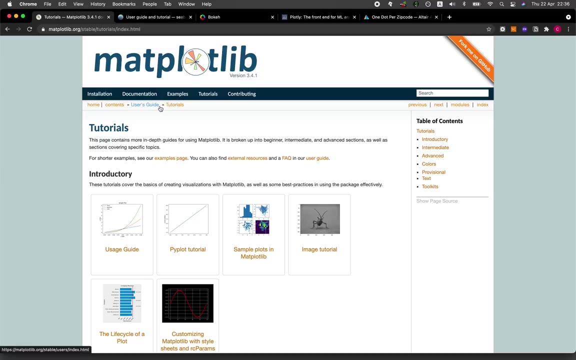 And it categorizes into different levels, like introductory level, intermediate level, Advanced, and also how to customize the colors. Okay, So both mapplotlib and Seaborn, they're quite similar in that the plots that you will create are pretty static, meaning that usually they're not interactive. 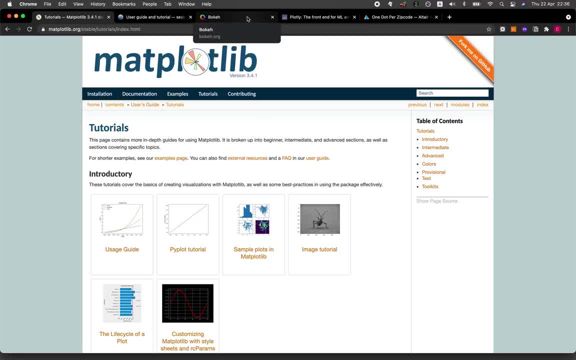 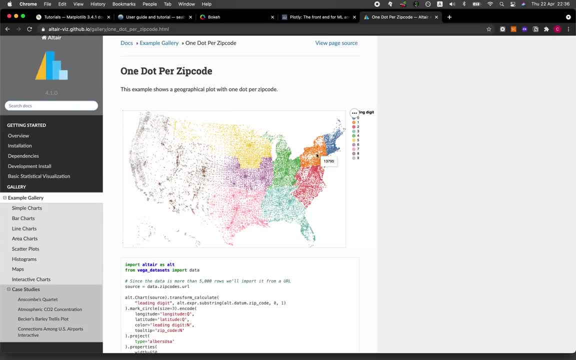 By interactive. let me show you what I mean. Let's have a look at Bokeh. So Bokeh, Plotly, and also Altair, they're interactive. For example, if I hover the mouse, you see that there is. 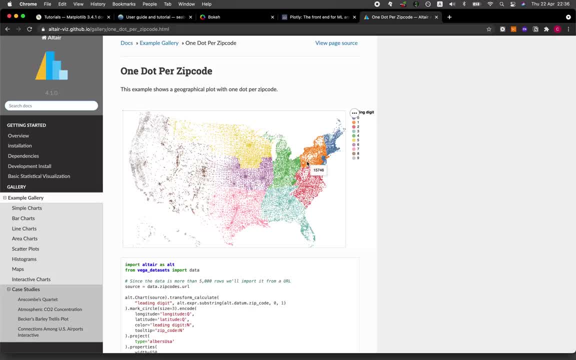 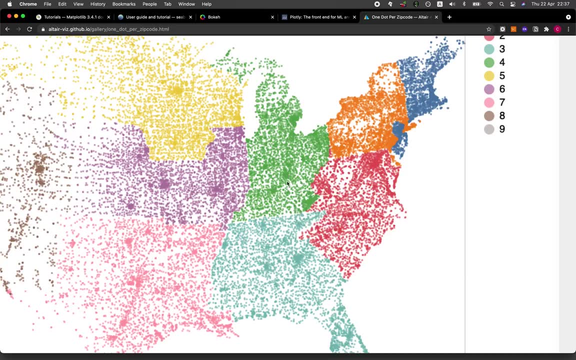 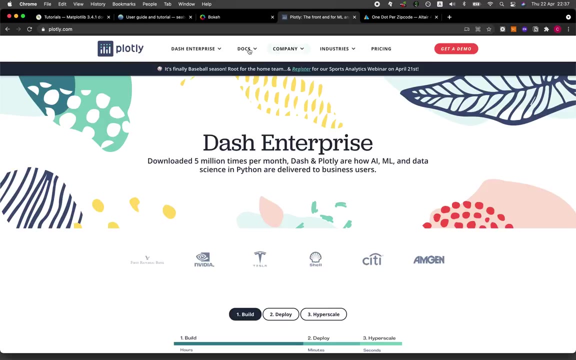 A number appearing: 15746.. If I change the hover to a new location, the number changes right: 41097.. If I move it again, the number updates Plotly also, let's have a look. So it's interactive charts. 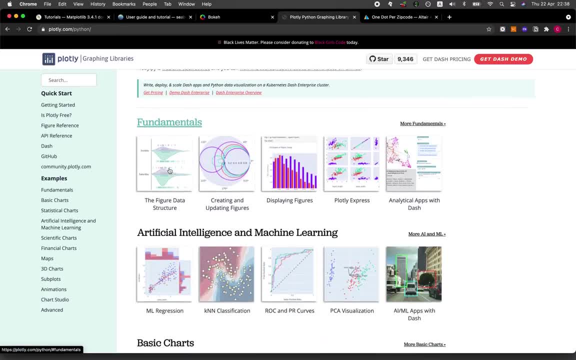 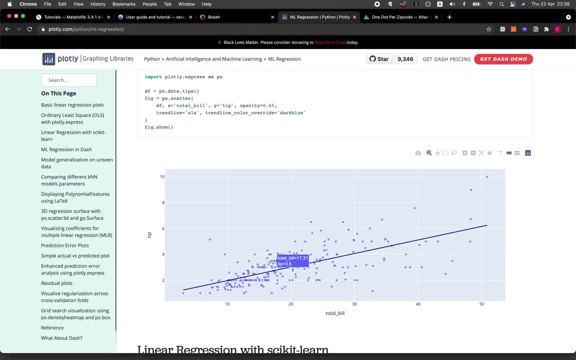 Let's have a look here. Let's click on one of them So you can see here that when we hover the mouse over a data point here we get to see the numbers displaying like total bill of 18.71 with a tip of four. 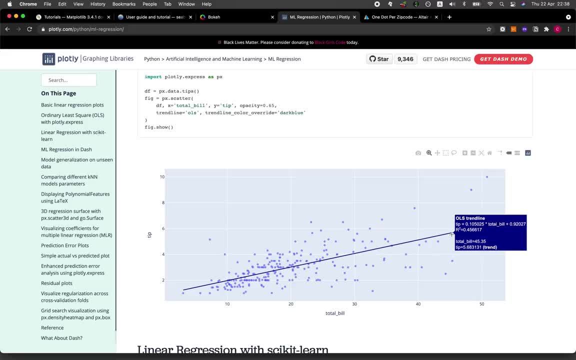 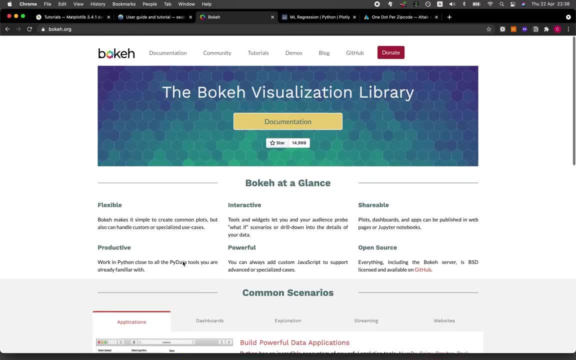 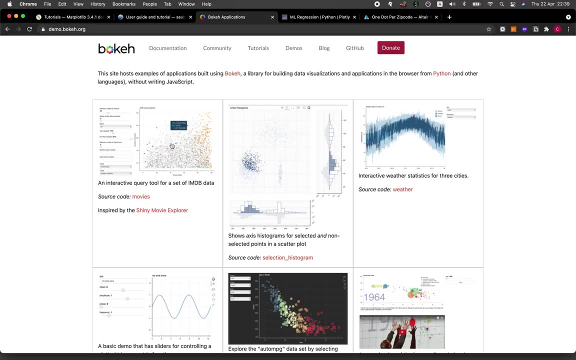 And it updates interactively, even on the line, the trend line here. Same thing with Bokeh. It's also interactive as shown in the examples here. Let's have a look at Some of the example plots, and right here it's quite amazing in that it looks quite a lot like Shiny. 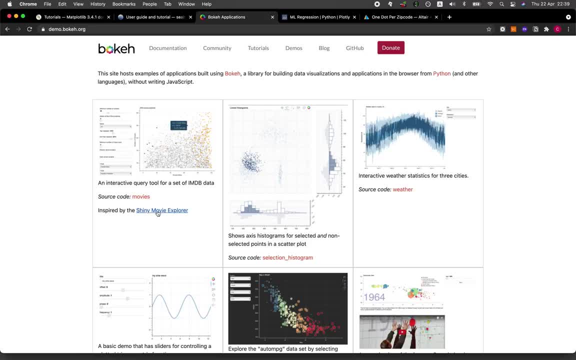 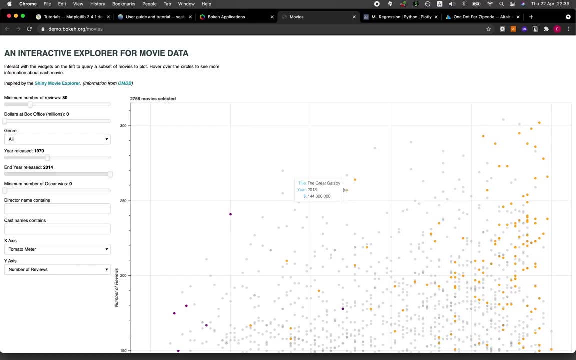 And, as you can see here, it's inspired by the Shiny example of the Shiny Movie Explorer. It's all of this resembles Shiny, the one from the data visualization package in R. Let's have a look. So if you hover on it, it updates itself. 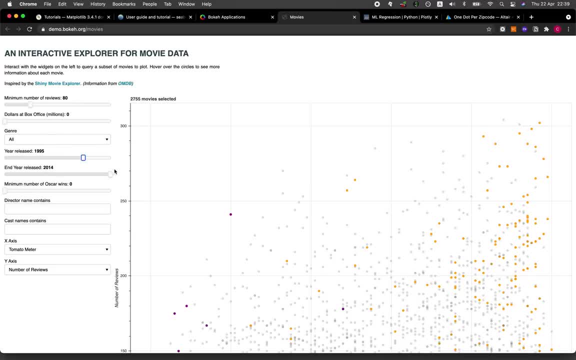 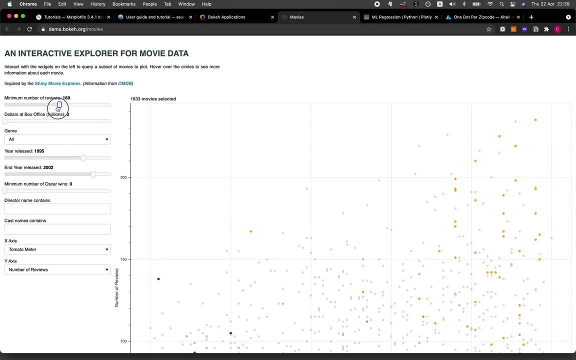 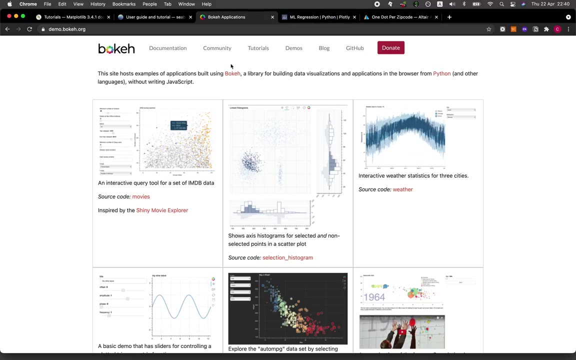 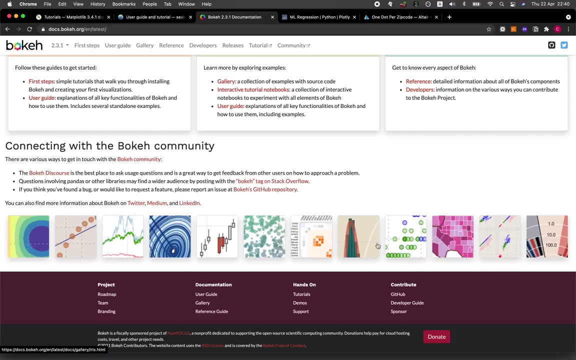 And the panel here is also interactive. So this is awesome. So you update here, the data gets updated. Okay, Let's have a look at the documentation. So there's a lot of different plots that you could make and they're all interactive. 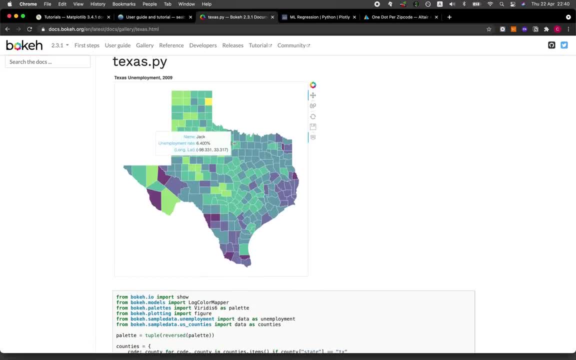 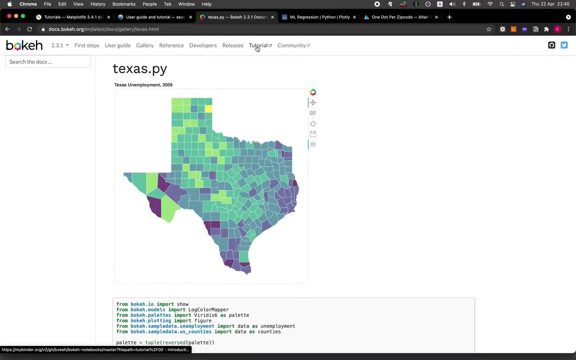 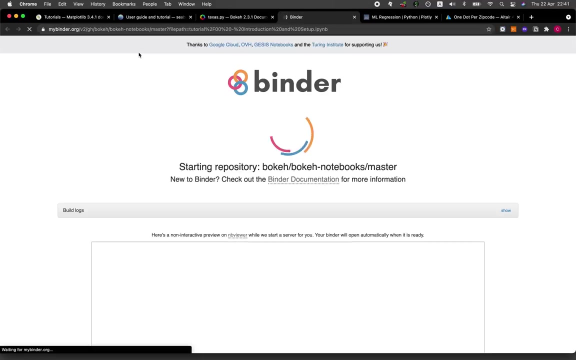 See, if you hover onto an area here You can get to see the name of the county updated for Texas and the corresponding is the example code. And they also provide you some tutorial as well. And it's linking out to a bender which will spin up a cloud notebook which will allow you to interactively use this Bokeh notebook. 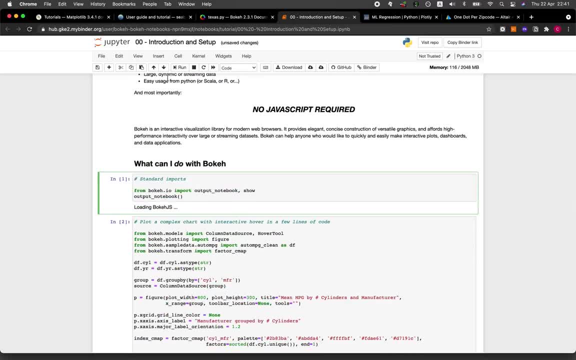 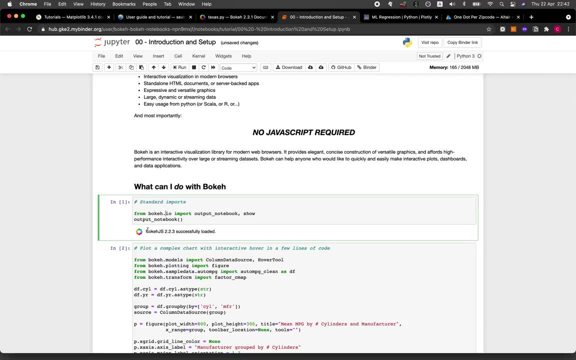 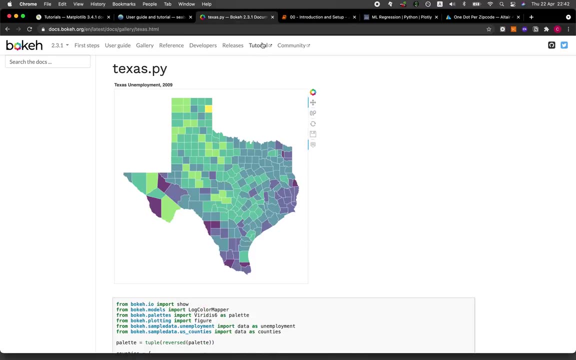 Let's have a look. It's loading up, loading Bokeh. Do I need to run it? It's fine, Okay, So it doesn't seem to show the example plot first to see. maybe it's loading, Oh well, So they do provide you with the tutorial, which should be interactive. 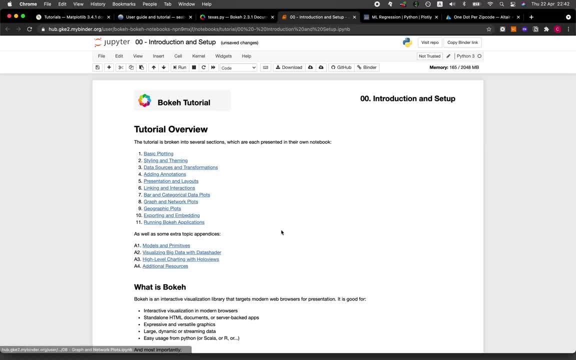 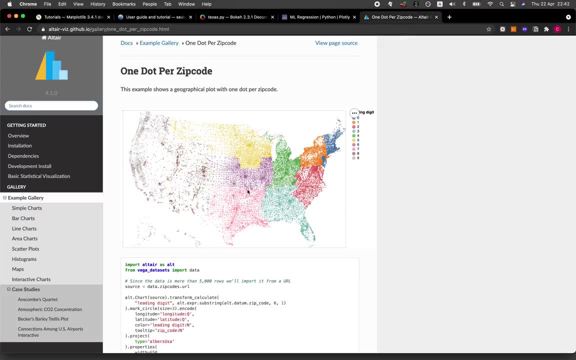 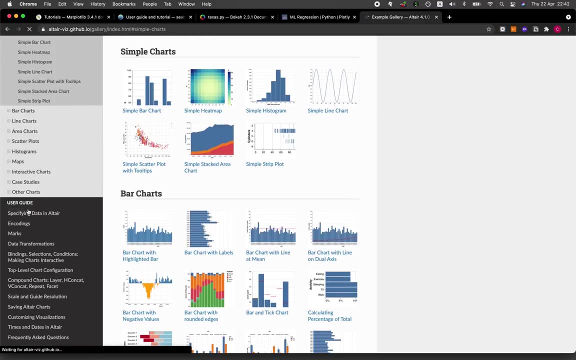 And so you could click on a topic of your interest and follow along in their tutorial. and let's have a look at the Out here. So this also another data visualization library in Python that is interactive and it looks quite good as well. Let's have a look at some of the example plots. So it's quite similar to mapplotlib in. 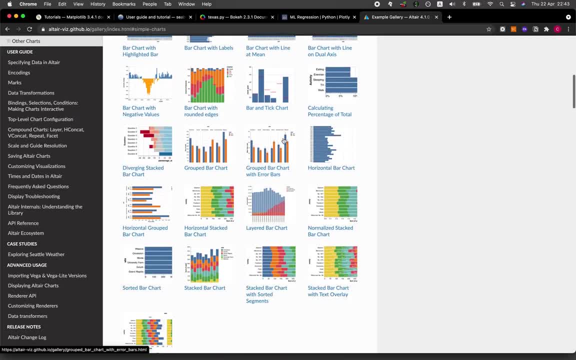 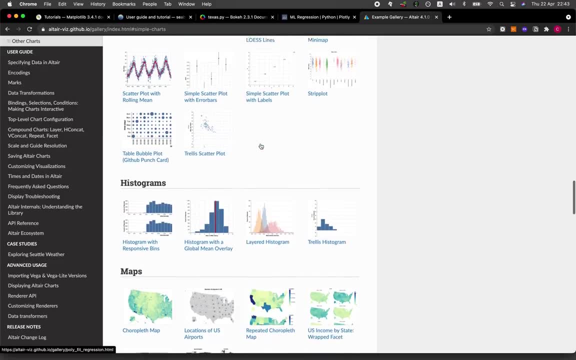 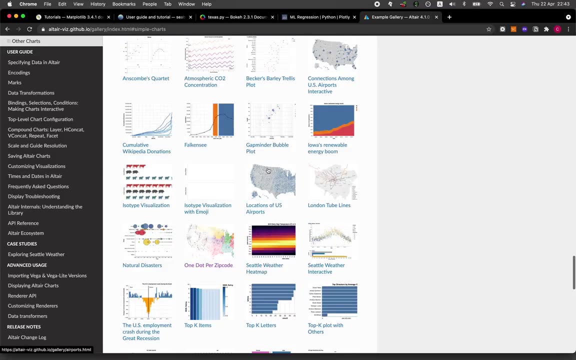 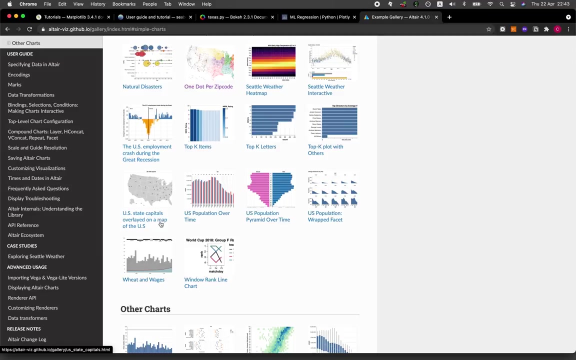 that it provides you a catalog of the example plots that you could generate- And the color is quite vibrant as well. Scanner plots, histogram maps- maps are pretty awesome here- Interactive charts as well, and also some case study examples. So they're pretty much the use of Altair in actual